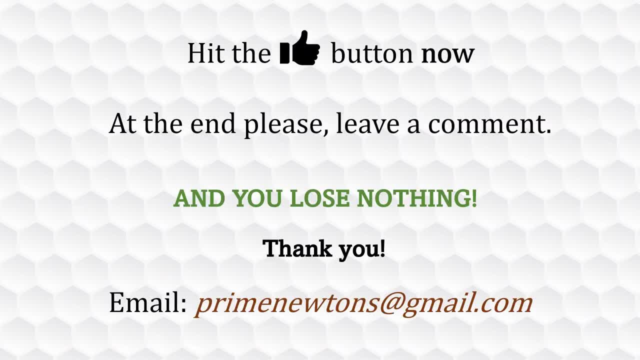 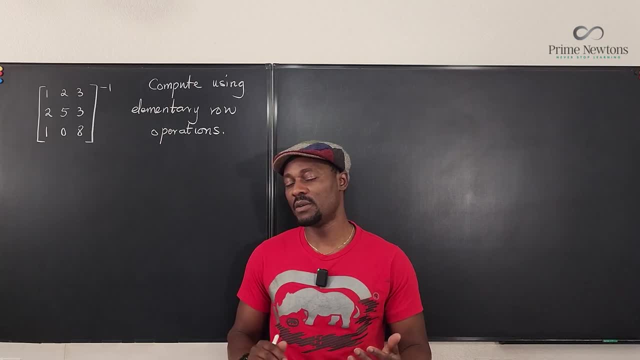 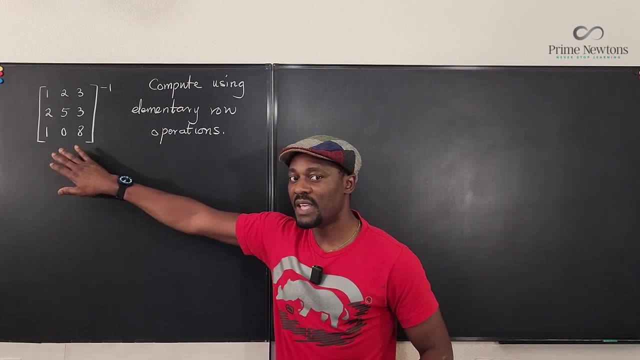 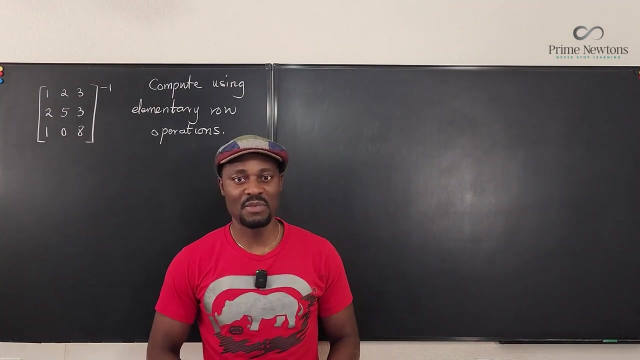 Welcome to another video, So let's continue our series on matrices and linear algebra. We're going to compute the inverse of this matrix using elementary row operations. I know we talked in the past about using the generalized formula for computing inverses, but from what I've noticed, 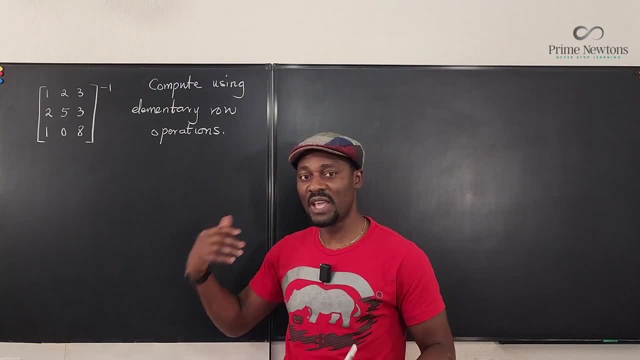 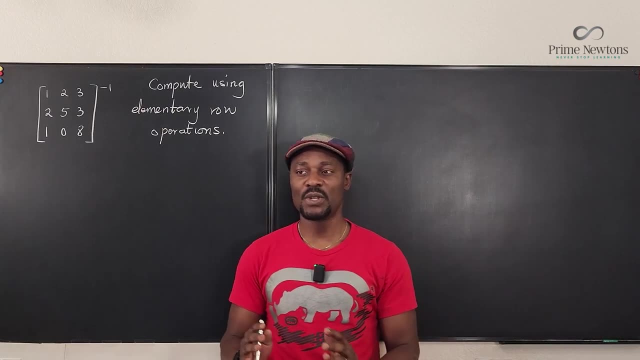 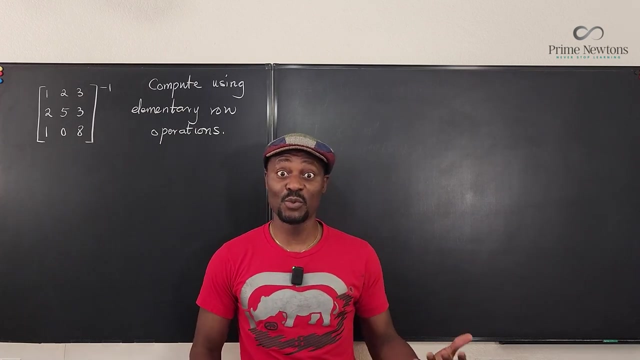 this is the most common strategy in computing: the inverse of a matrix. So let's do it, And all you're doing is you will make an attempt to convert the identity matrix for a three by three into something else, which will end up being the inverse matrix, And you do that while you're. 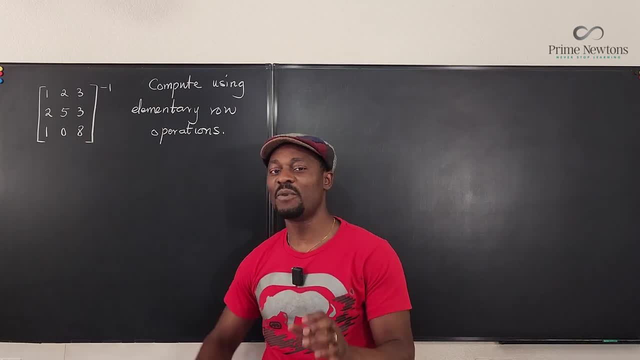 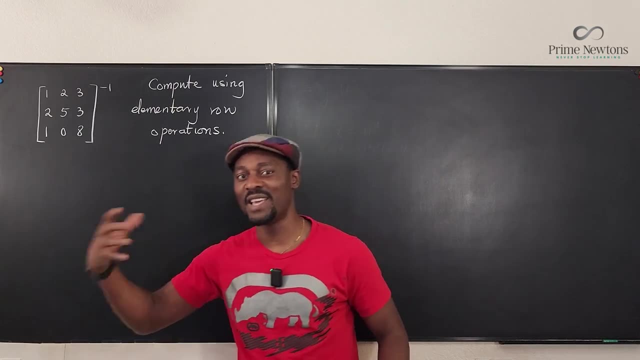 trying to compute the inverse of a matrix. So let's do it, And all you're doing is you will to convert this into the identity matrix for the three by three, So you put them side by side. you work on this while you are simultaneously working on the identity matrix. So by the time, 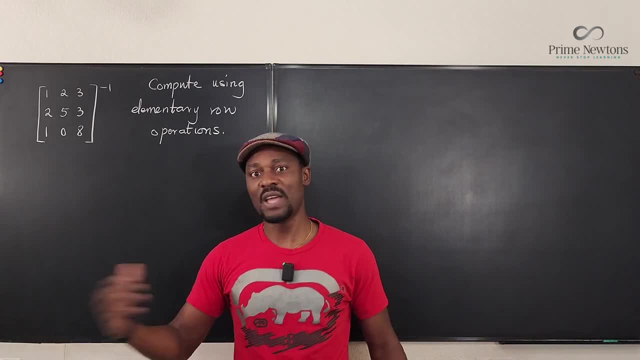 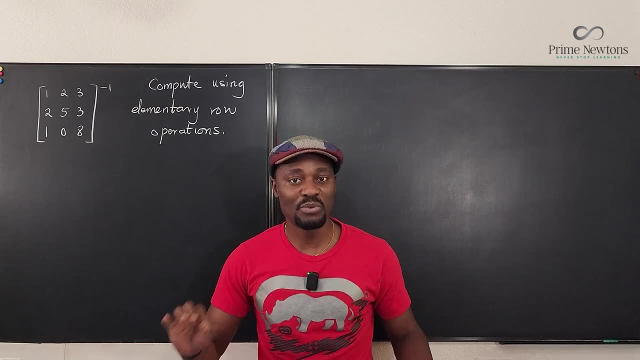 you do everything to change this into the identity matrix, then you have the inverse matrix. Okay, now what is the problem with this method? There is zero problem, except you're more likely to make computational errors while you are subtracting. So let's do it And all you're. 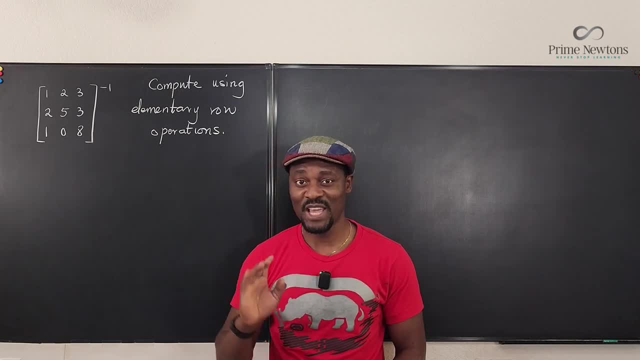 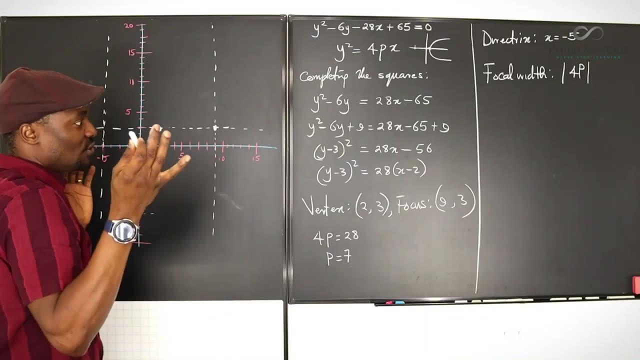 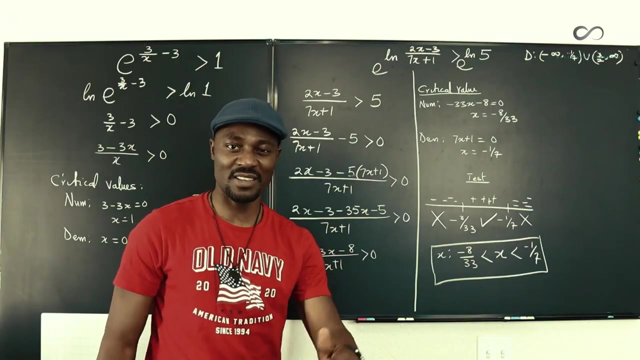 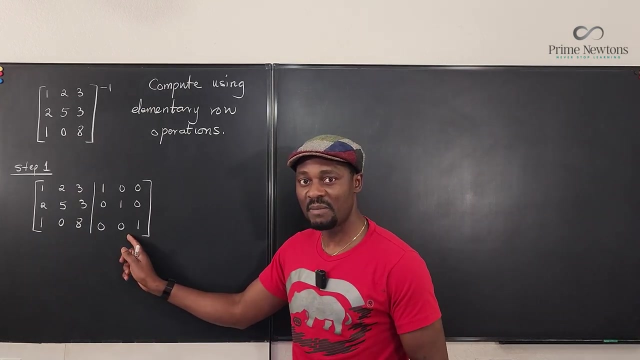 doing is you're subtracting or adding the rows together to get your zeros. So let's get into it. So the very first thing that you do is write both matrices this way. This is the identity matrix for a three by three, And this is the matrix you're trying to invert. So what you're doing is you're. 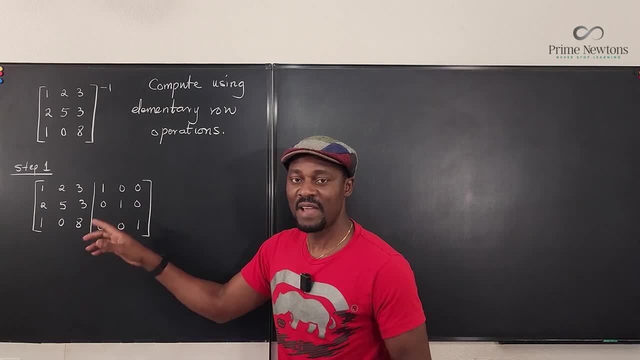 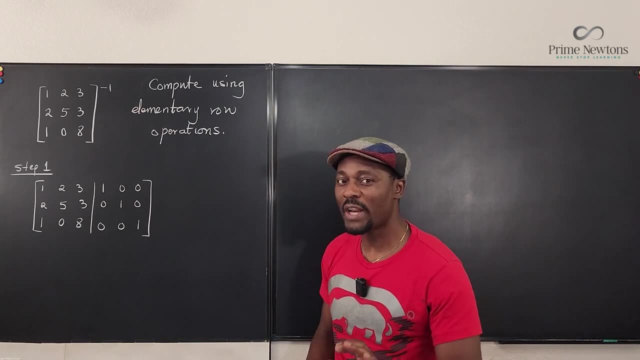 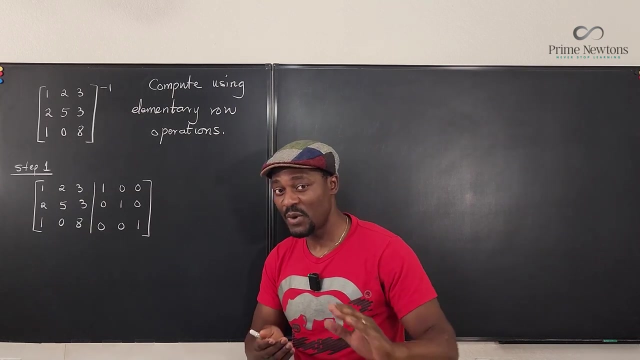 going to make this look like this And eventually this is going to look different And whatever is on the right hand side becomes the inverse matrix. Okay, so what can you do And what is the best strategy? You want to go the way of the row echelon form, which means you want the very first. 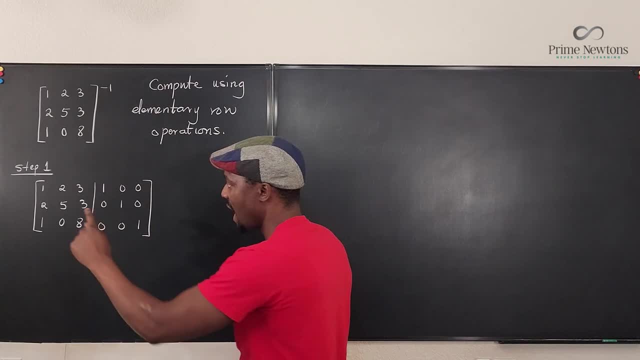 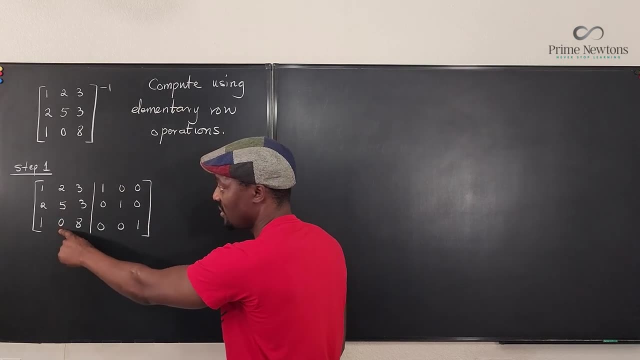 number here to be one and everything under it to be zero. the very first number here to be one and whatever is here should be zero. This is a good zero, but we still have to muddle things up a bit. You want this also to be one? 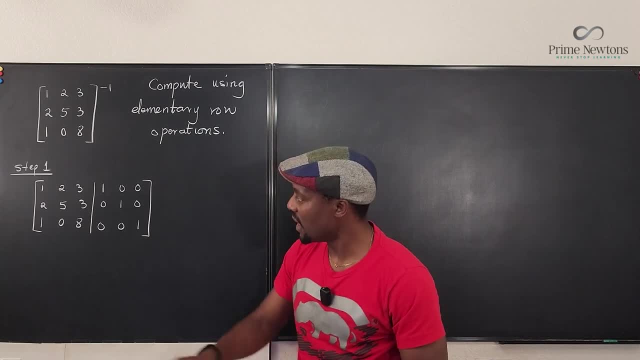 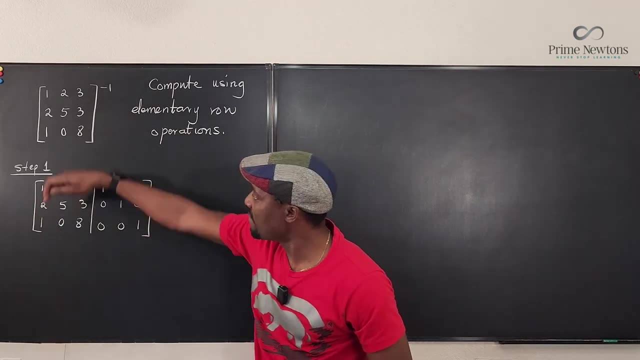 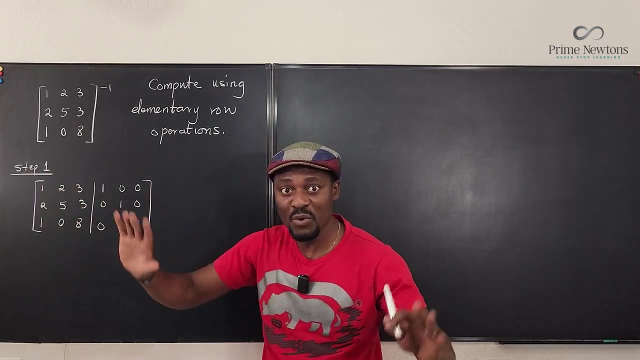 And then we can take care of whatever is above. So what you want to focus on is anything under this first thing. here you want to make it a zero. Now we have a very good matrix, because the very first entry is a one. If it was not a one, and the one was this one, your first move. 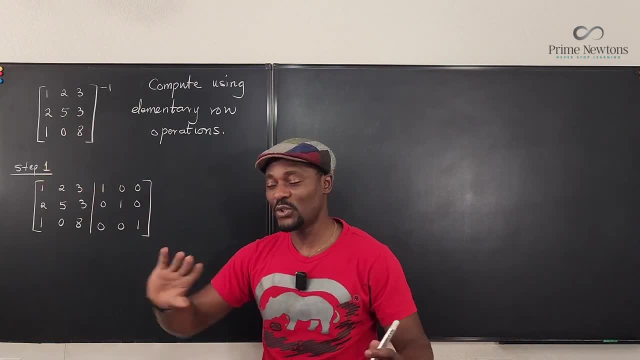 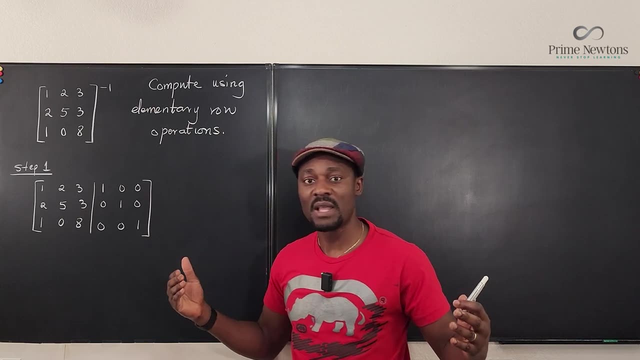 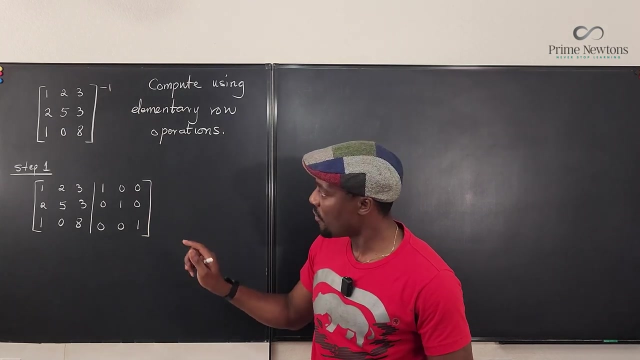 would be to switch it. Okay, instead of you starting to divide, just switch them and have a one on top. It's easier to work with one because you can multiply and add or subtract easily. So, first move we're going to make- I think I'm going to write the instructions here, First move I'm going to make. 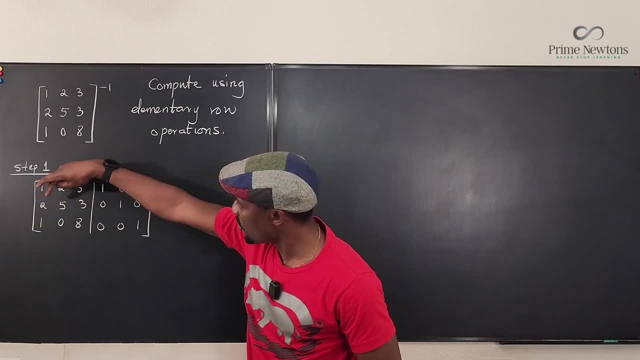 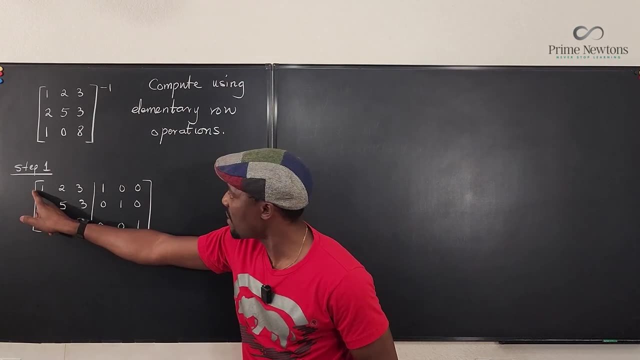 is to get zeros under this first one. So I will say I am going to add minus two of row one. If I multiply this first row by minus two and then I add it to this, I'm going to get a zero here. 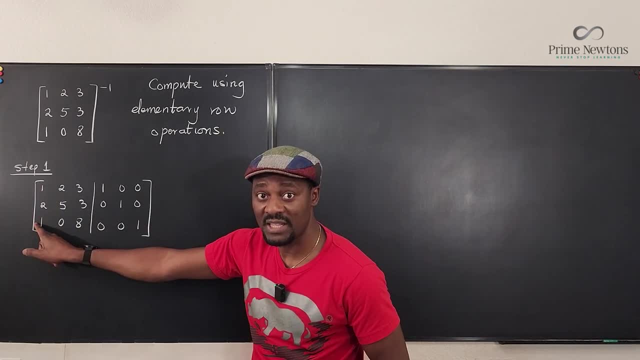 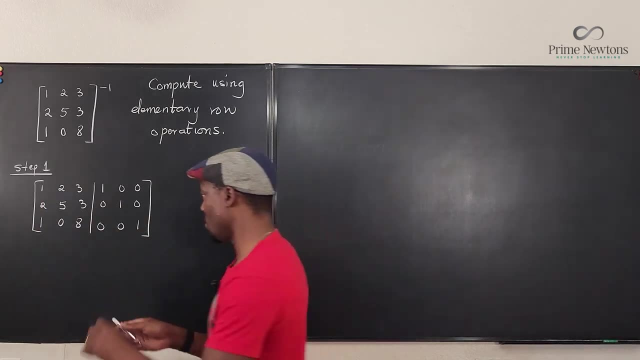 If I take minus of this and add it to this, I'm going to get a zero here. Now don't focus on anything else, Just focus on this, because that's what saves you. So, instructions: we're going to say that the new row two. 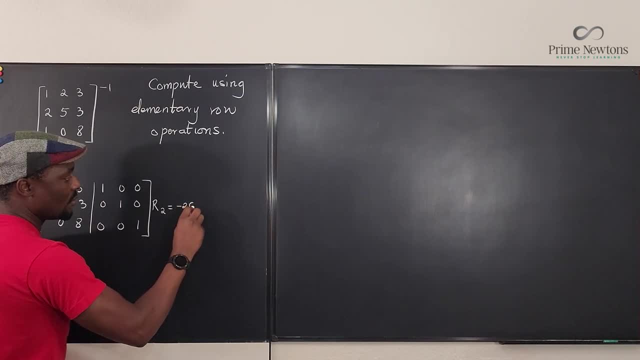 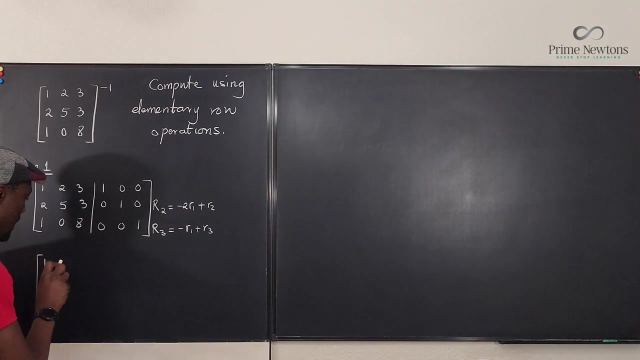 is going to be minus two of row one added to row two, And then the new row three is going to be minus row one added to row three. That's what we're going to do. So let's have the next matrix. This is going to be because we're not modifying the first row. always copy the first row One. 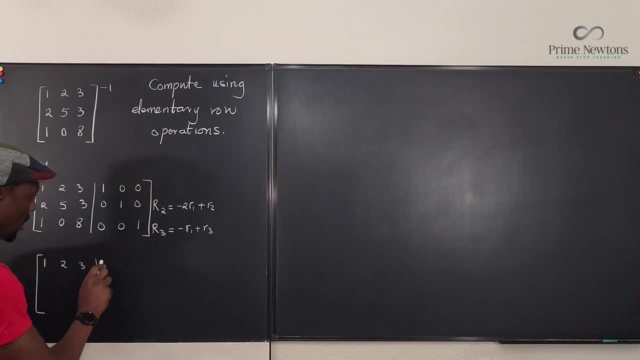 two, three. So the row you're not modifying, just copy one zero, zero. Okay, we're modifying the second row. It means you're guaranteed to get your zero here, Okay. so now let's finish this. Minus two times, this is minus four. If you add minus four to five, you're going to get one. 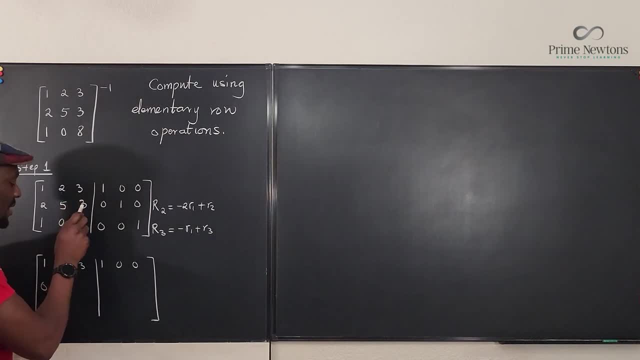 Minus two times this is minus six. If you add it to three, you're going to get minus three. We're going to keep going. Okay. minus one times two is going to be minus two, And minus two added to zero is minus two. Minus two times this is zero. added to this is one Minus two times zero. 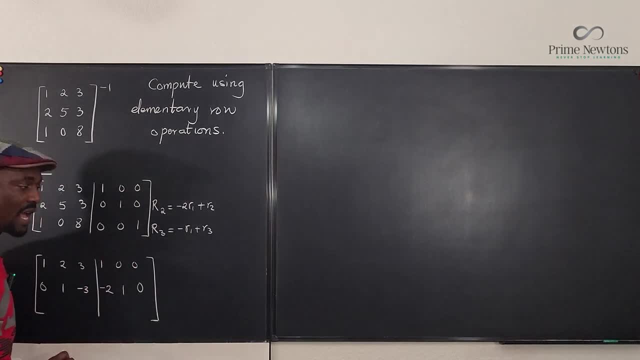 is zero. added to zero is zero. So we're done with that. Let's go to this one. This is going to be minus row one plus row three. So it's going to be minus one plus one. we get zero. We're going to have minus two. sorry, we're going to have minus two plus zero. 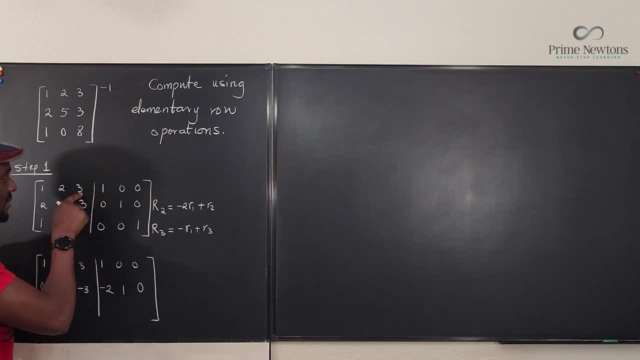 is going to be minus two, And we're going to have minus three plus eight, it's going to be five. Nice, We go here. we're going to have: minus one plus zero is minus one, minus zero plus zero is zero, and minus zero plus one is one. So we're done with the first one. This is the first move. 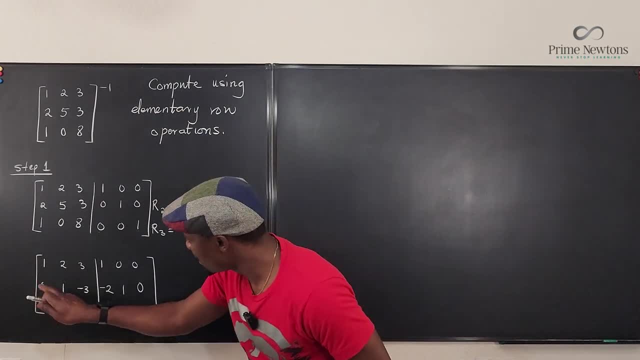 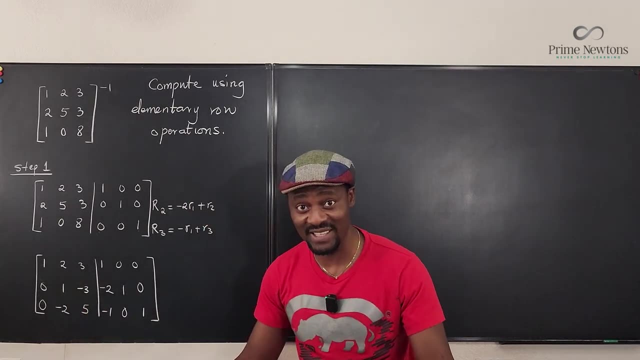 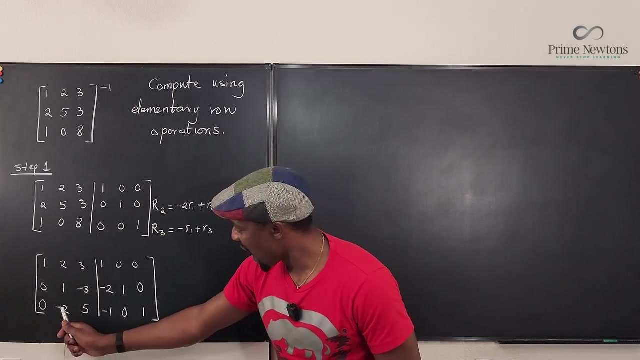 where we are Next thing. we've attained zeros under this one, And nicely. we have a one here, So we don't need to worry about this second one. It's a very easy example, But we need to create a zero here. That's the next zero mission. Okay, so how do we create a zero here? Well, add two of 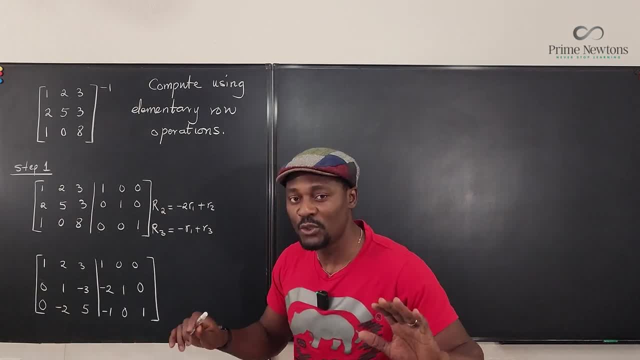 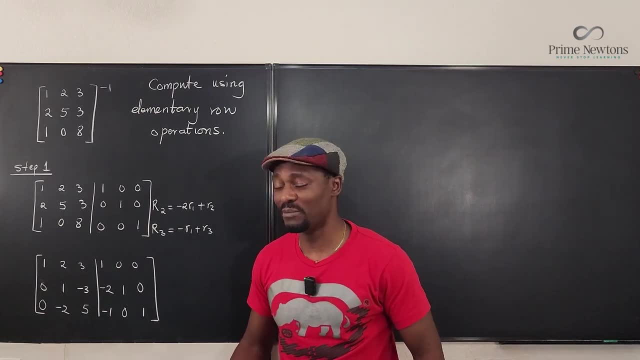 this to this, you're going to get a zero. That's our next move. Okay, don't rush, don't double things. That's what I did. I made so many mistakes, got my answers wrong, failed so many quizzes and tests, just because I was always trying to do too many things at the same time. 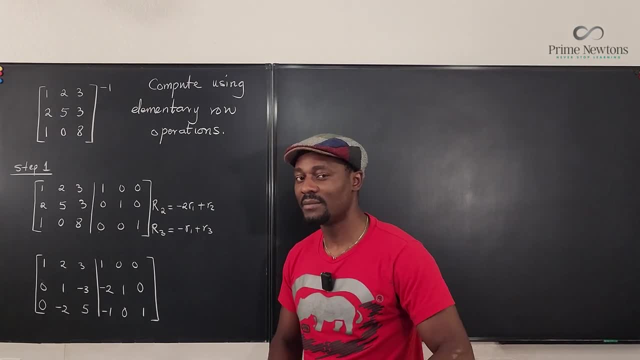 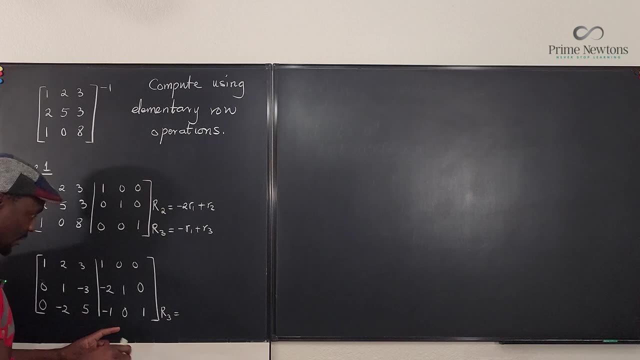 When you get used to it, do it, But when you're still learning, don't try it at home. So we're going to say that row three, the new row three- because we want to make a zero here- will be just two of row two added to row three, Two of this added to this. we're going to get an answer. 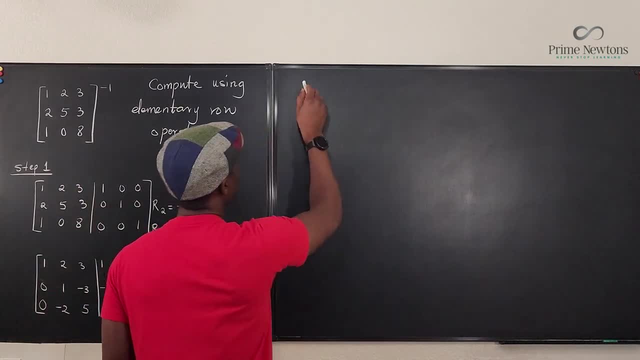 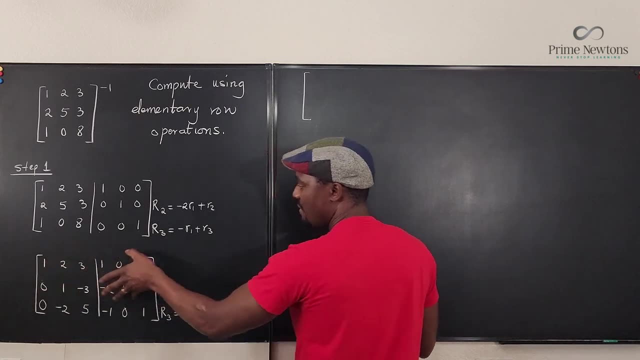 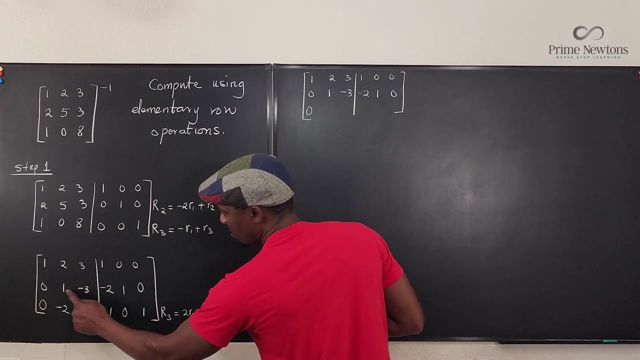 So let's see what we get. So here we're going to have, because we're not changing this and we're not changing this, let's copy everything in the first two rows. So two of this plus this gives me zero. Two of this will be two minus two, that's. 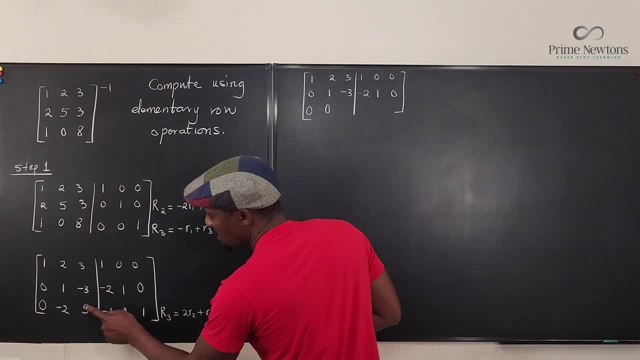 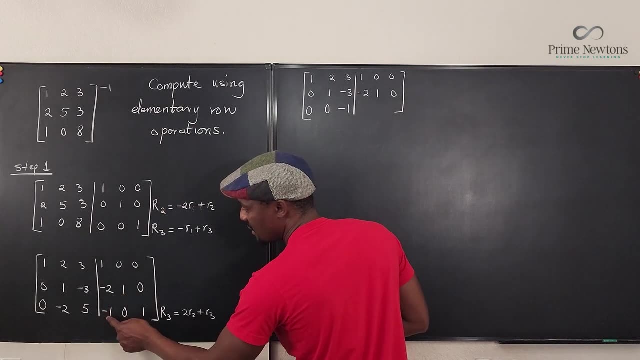 zero. Two of this is minus six. If you add it to this, it would be minus one. Let's go. Two of this will be minus four. If I add it to this, it would be minus five. Two of this will be two. Add it to zero. you get two, And two of this will be zero. Add it to one. 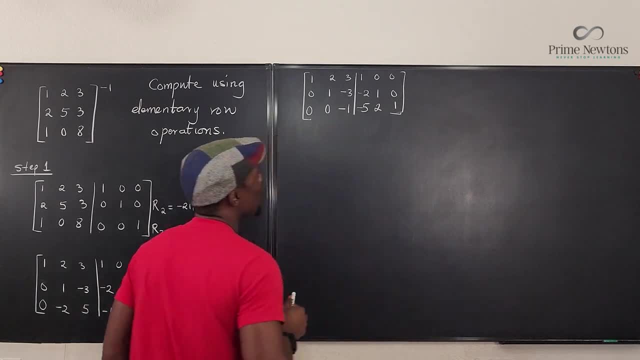 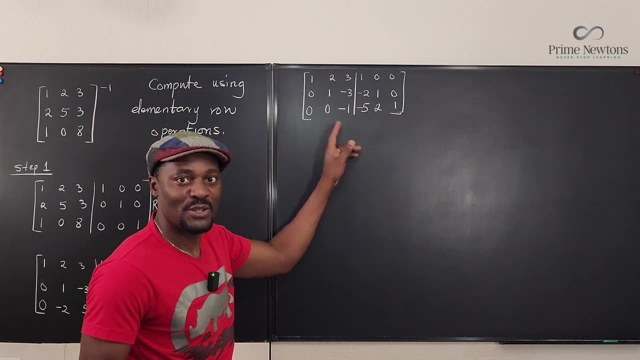 you get one. Okay, so that's our new matrix. What can we do again? We need a one here, We don't need a zero. And this is easy to change: minus one to one. You just multiply by a minus one, So we're. 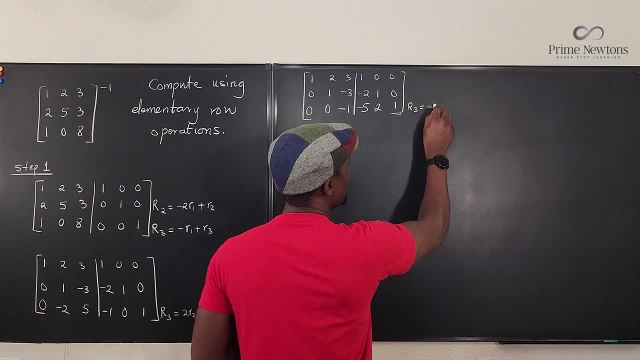 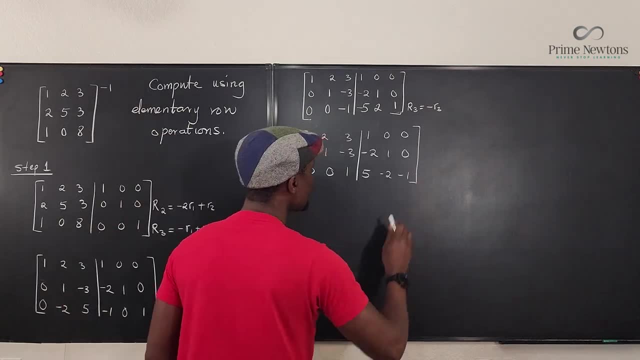 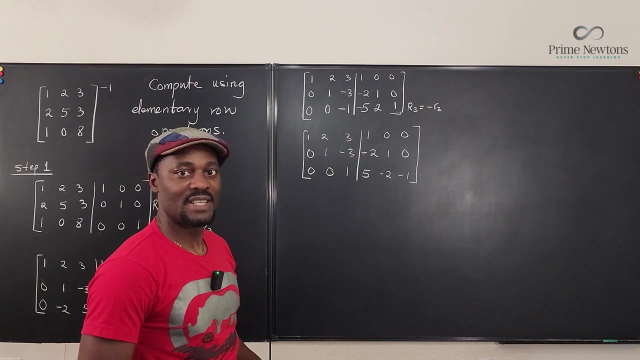 going to multiply this. The new R3 is minus the old R3.. Okay, let's write it down here Step by step. So what can we do Now? nothing here should be anything. We want to get rid of these guys here and we want to get rid of this also, But you shouldn't do it together. 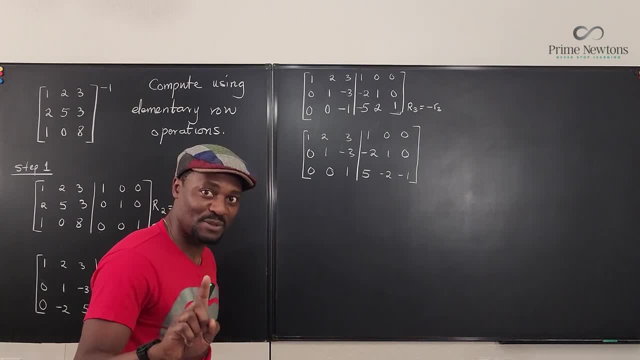 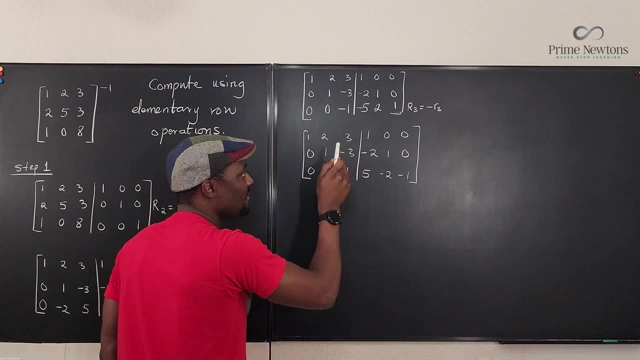 That's the mistake I always make, Okay, so don't make those mistakes. Be smart. We're going to try to eliminate these. Okay, what do I do? I'm going to add three of this to this, and I'm going to. 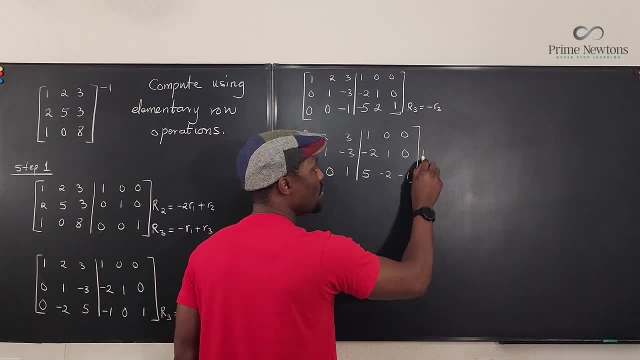 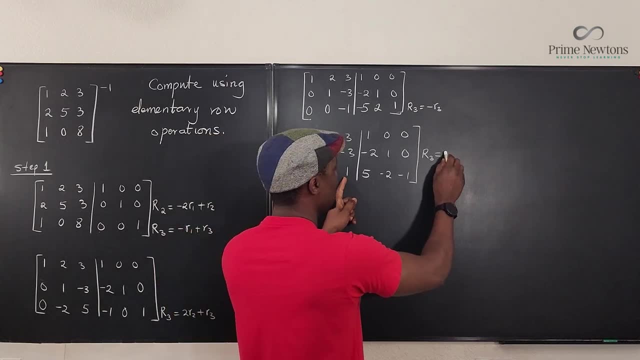 subtract three of this from this. So I'm modifying R3.. So I'm going to say R3.. R3 is the old R3.. Okay, it's going to be three of R3 added. Sorry, this is R2.. Added to R2.. 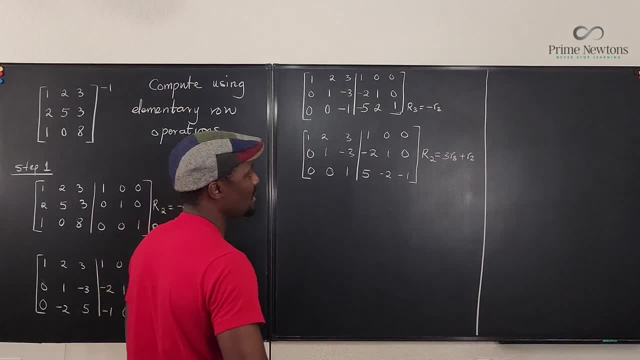 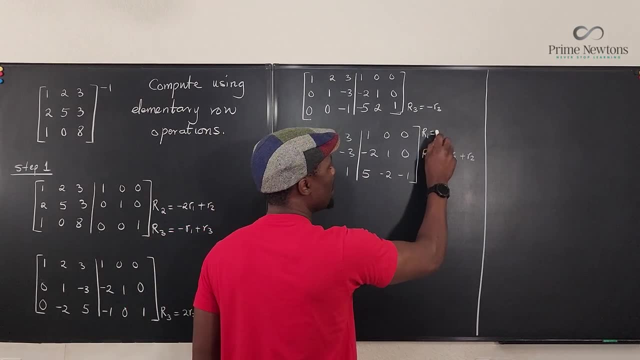 Need to make space for the last few ones we're going to do. And then for this one, it's going to be three of this subtracted from this. So R1 will be equal to three of old R3 subtracted from this. So it's going to be minus three of this. So let's go here: Minus three, R3 plus R1. 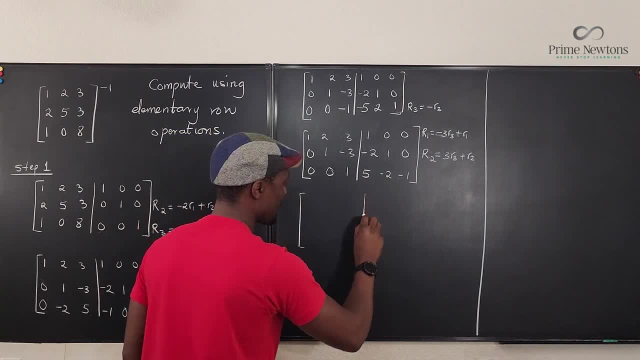 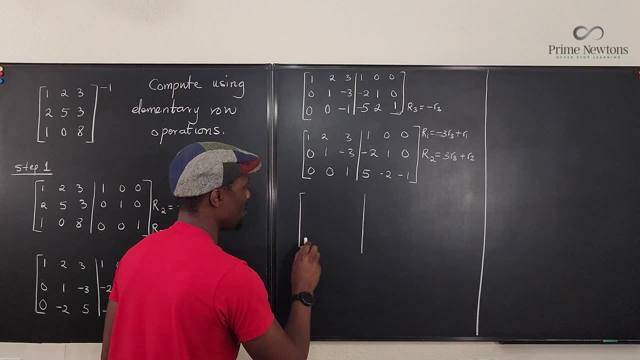 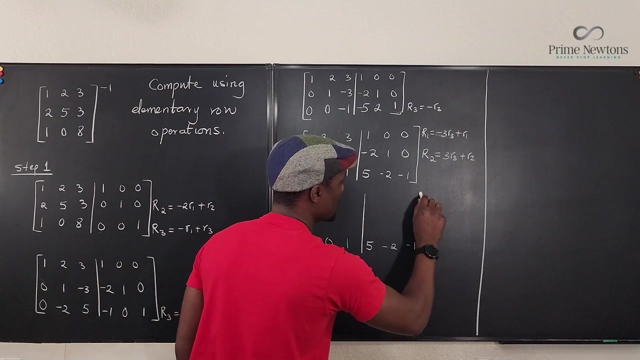 So this is going to be three of this. added to this, That's going to give us zero. Which one are we not modifying? We're not modifying the bottom one, So let's just copy Zero, zero, one. five minus two minus one. We need three of this. added to this, It's going to be zero. 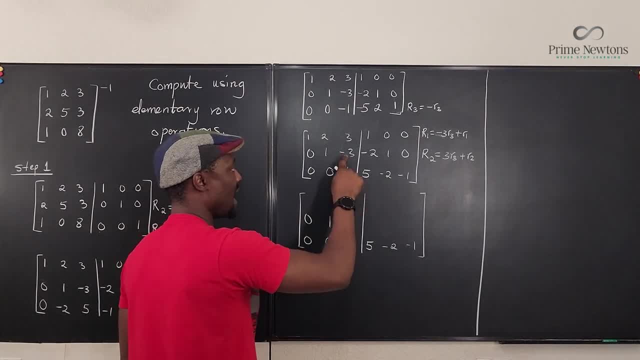 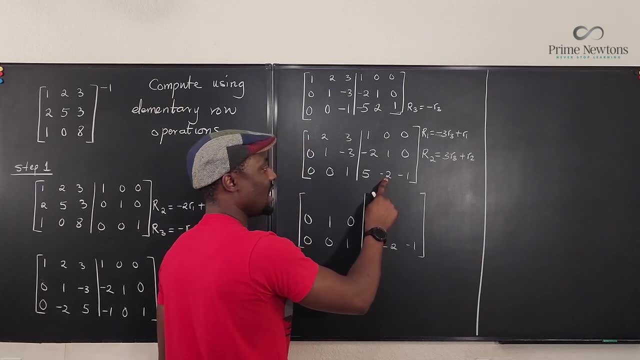 Three of this, added to this, is going to be one. Three of this, added to this, is going to be zero. Three of this is 15.. Added to this, is going to be 13.. Three of this is minus six. Added to this is: 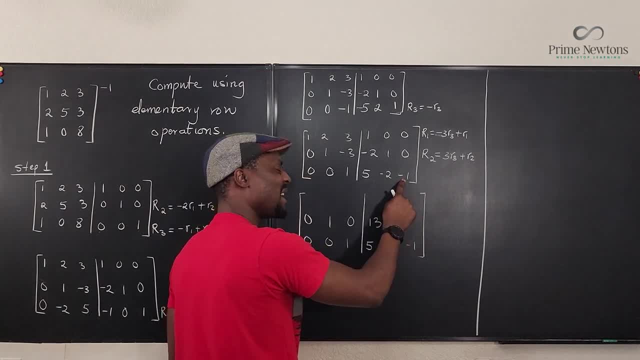 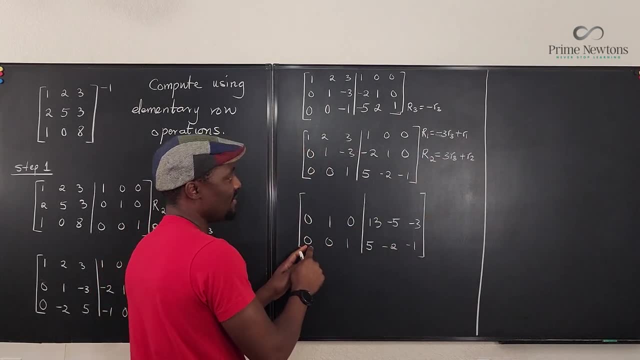 going to be minus five. Three of this is minus three. Added to this is going to be minus three. Okay, let's go here. It's going to be minus three of this. Okay, minus three of this added to this. So that's just one. 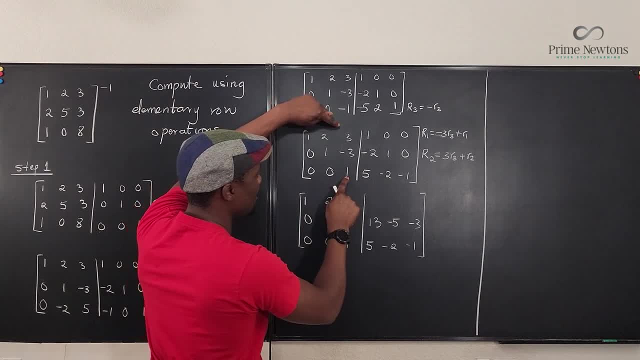 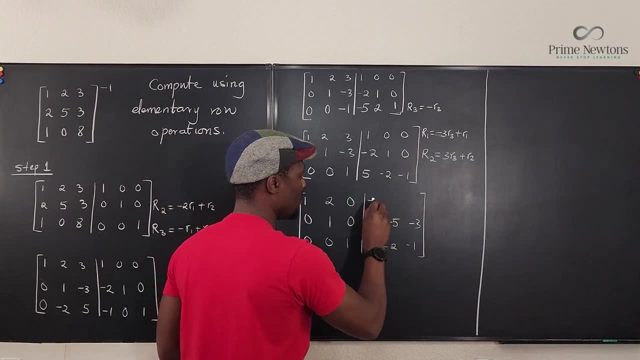 Minus 3 of this, added to this, is just 2, and minus 3 of this, added to this, is 0.. Minus 3 of this is minus 15,, added to this, would be minus 14.. Minus 3 of this is going to be 6,, added to this, you get it to be 6.. 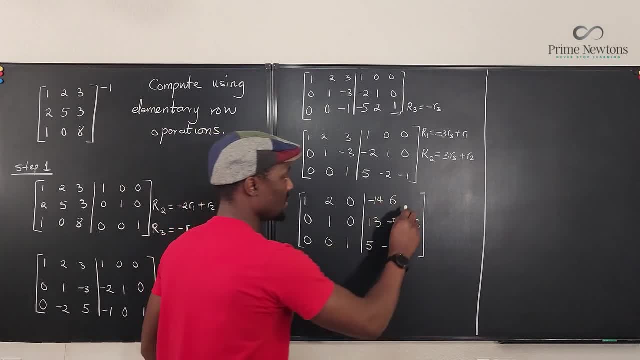 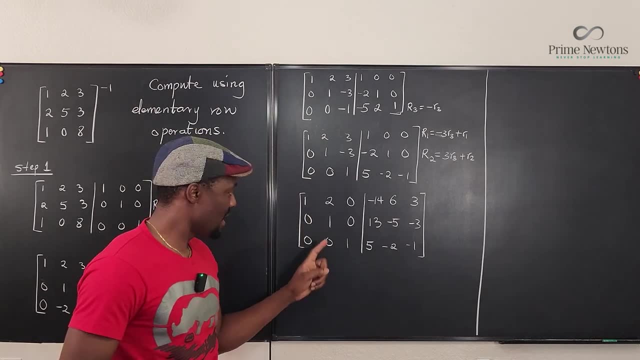 And minus 3 of this is going to be 3.. So that's what we have. The only thing remaining one more move is just to get rid of this guy here, And we can do that by doing minus 2 of this added to this, and then we're done with the answer. 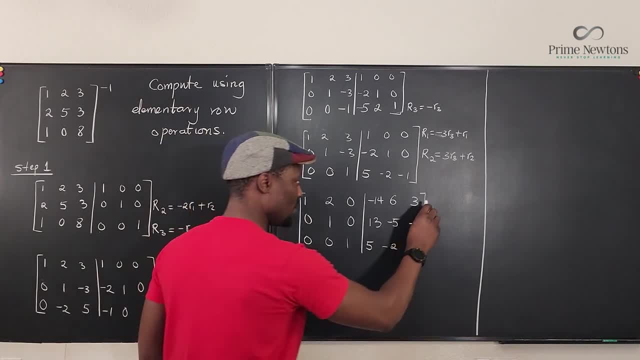 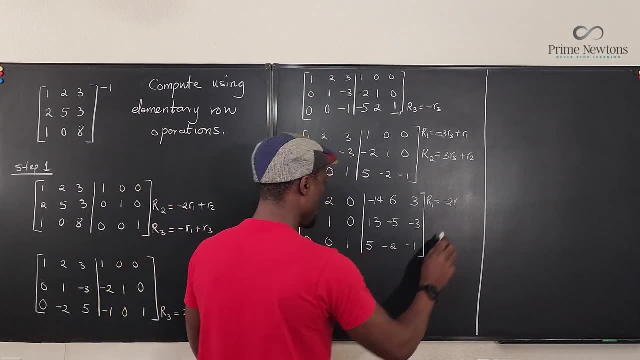 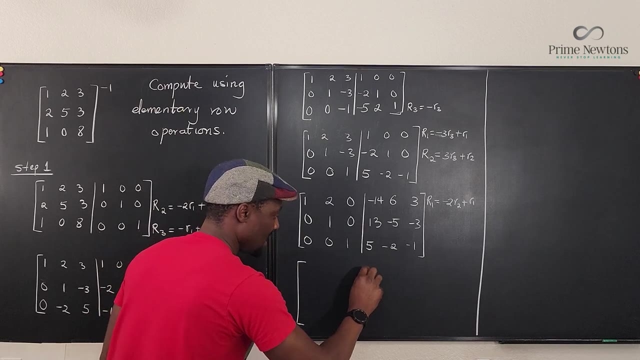 So this is the only line that needs to be modified. So this row- row 1, will be equal to minus 2 of the old row 2 added to row 1.. Okay, let's see how that turns out, Nice. 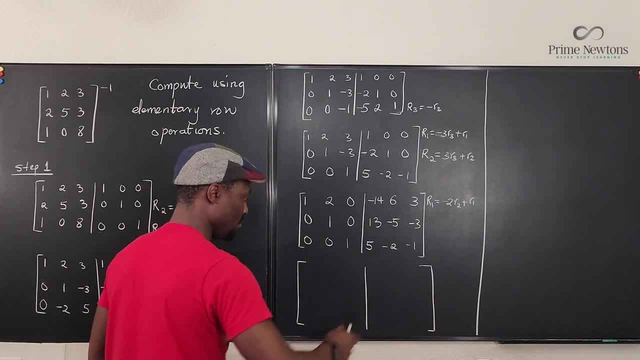 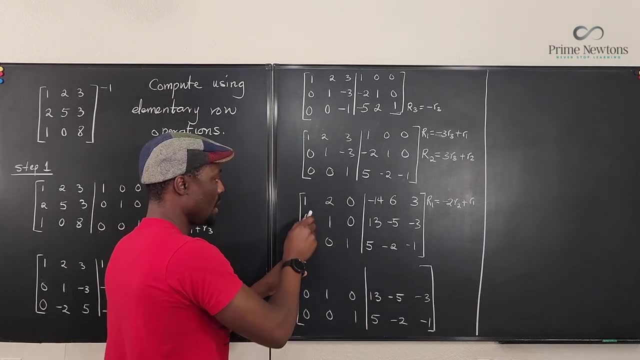 So, as you can see, we're not modifying the bottom 2 rows, So I'm just going to copy the bottom 2 rows minus 1.. Okay, so let's deal with this: Minus 2, row 2, plus row 1, that still gives us 1.. 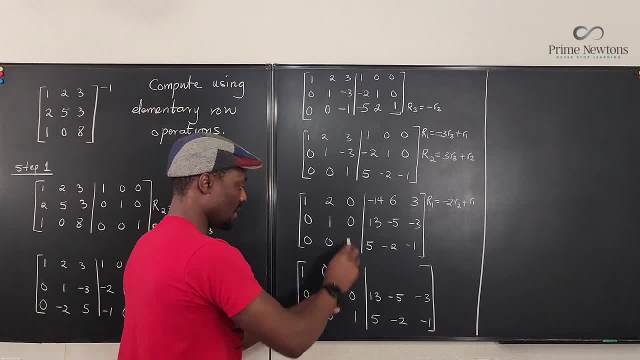 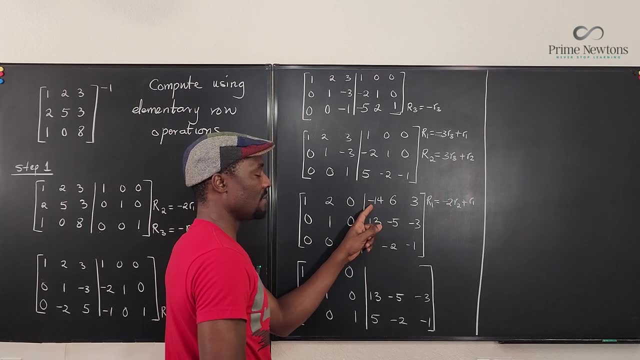 Minus 2, row 2, that gives us 0.. Minus this is still 0,, so let's go here. Minus 2 of this is going to be minus 26,, minus 14,, that's minus 40.. 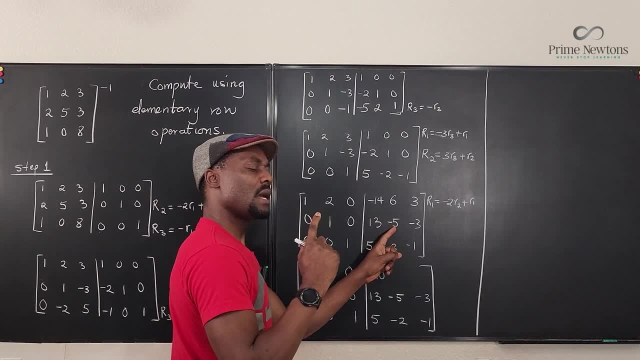 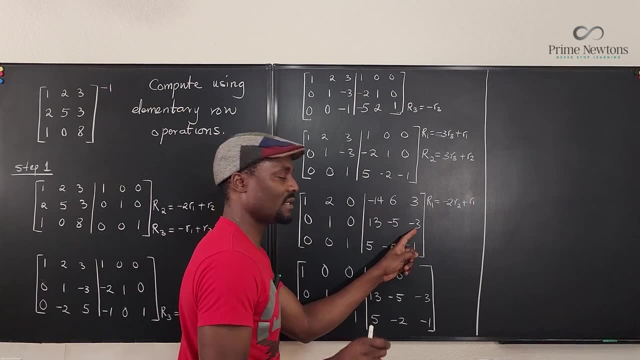 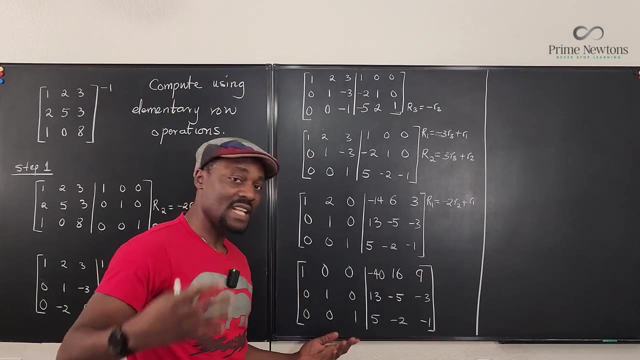 And minus 2 of this would be 10, plus 6.. That's going to be 16.. And minus 2 of this is going to be 6, plus 3, that's going to be 9.. Okay, so you see, we have generated the identity matrix for a 3x3 on the left-hand side. 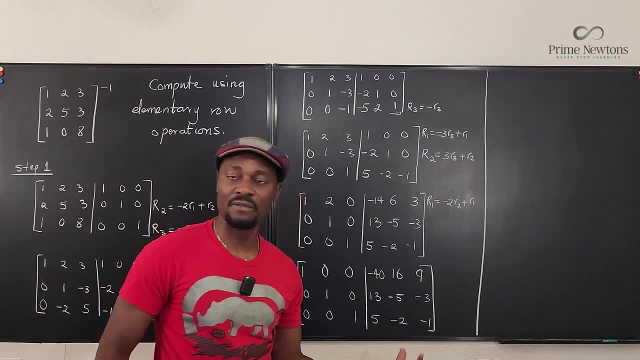 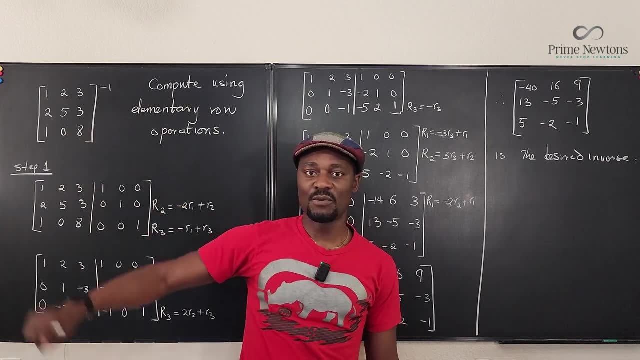 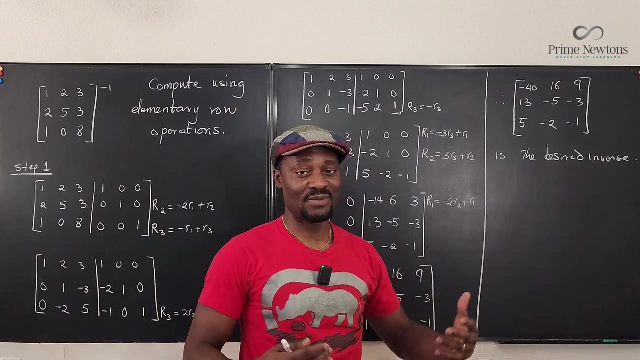 Automatically. if all your work is correct, this is the inverse of this matrix, So you can say that this is the desired inverse, that we wrote this way. Now, this has a bunch of integers. okay, Most of the time they're fractions. 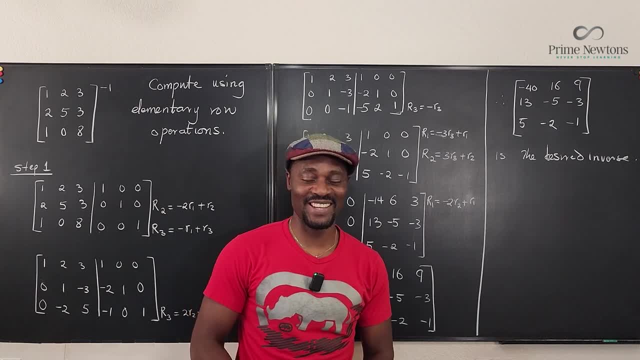 You have to be ready to deal with fractions. See you in the next video. Never stop learning. Those who stop learning have stopped living. Bye-bye.